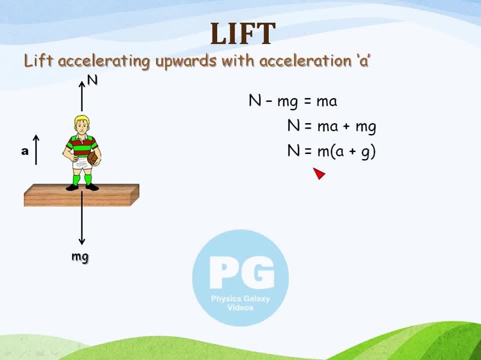 Of course, if we talk about the net force in the direction of acceleration, we can say it as n minus mg is equal to mass into acceleration. Simplifying this equation, we can write mg And as here. so we can write normal is equal to m, a plus mg. So if it take the mass common, we can write m into a plus g. Note that weighing machine majors the normal reaction of a person. 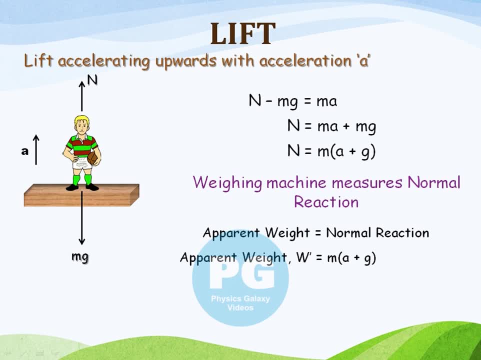 That is the apparent weight of the person i, and the lift is equal to the weight of the person i. So the apparent weight we denoted by w dash that is equal to the normal. that is m times a plus g. So if we take here g as common from this we can write mg Bracket a upon g plus 1.. 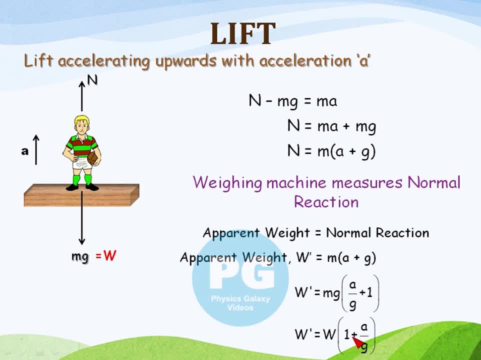 This mg is what the true weight that we denoted by symbol w And we can rewrite the apparent weight as w 1 plus a upon g. Thus the person true weight is not changed, but his apparent weight has changed. Thus the person true weight has increased by an amount equal to m a. 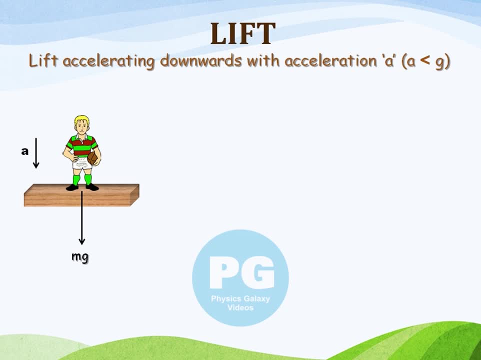 Now when elevator is accelerating downwards. Thus again, the two forces acting on the person is mg in the downwards and normal force upwards. In this case, the net force acting on the person is downward and normal force is less than the true weight of the person. 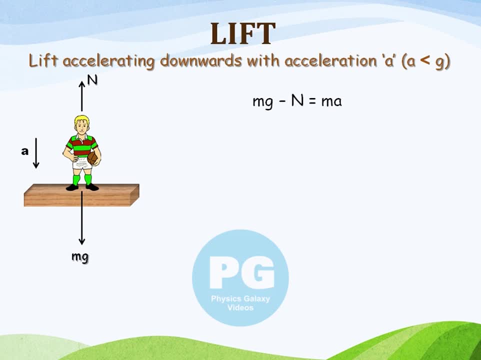 So if we apply Newton's second law in this case We can write the net force acting on this person In the direction of acceleration as mg minus n, So mg minus n is equal to mass- into acceleration. So here if we write the normal reaction gives mg minus m a. 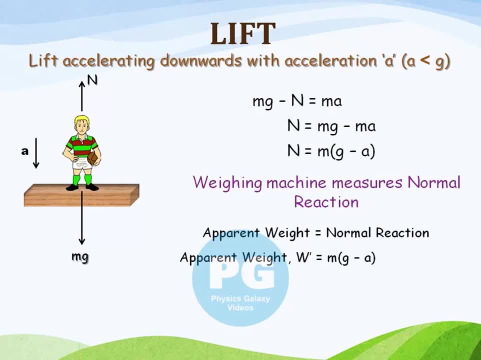 So if we take m as common, we can write: normal force is equal to mg minus a. Again, note that the weighing machine majors the normal reaction. So if we say the apparent weight is equal to the normal reaction, That means the apparent weight, that is w dash, is equal to m. 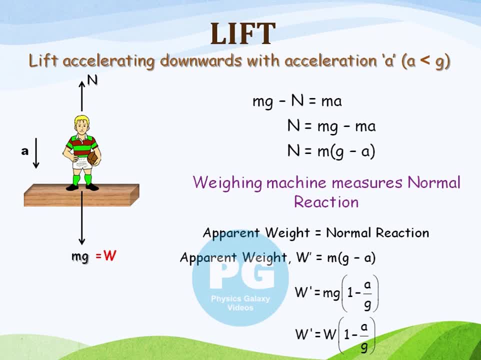 Times 3. Minus a. If we take g as common from this equation, we can write mg in bracket, 1 minus a upon g. The mg is what The true weight. So we can write the apparent weight as w 1 minus a upon g.